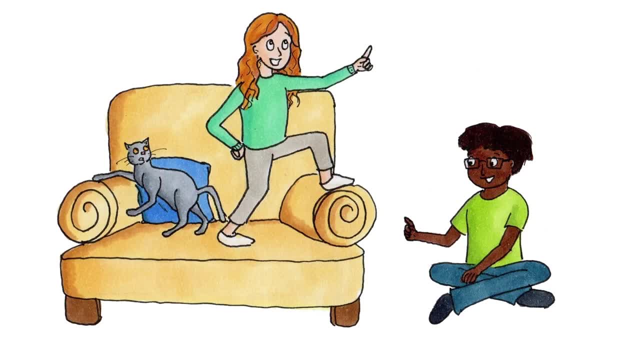 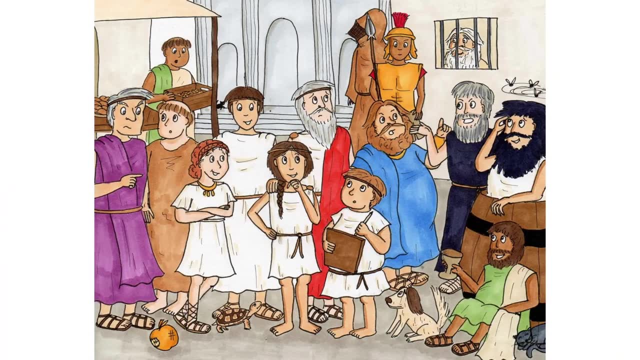 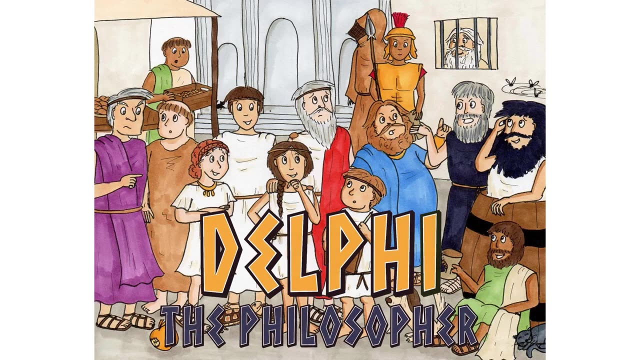 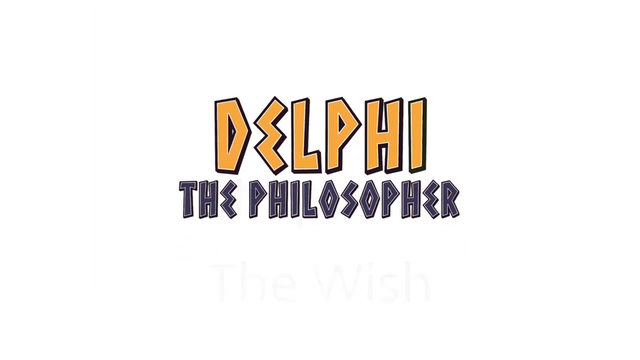 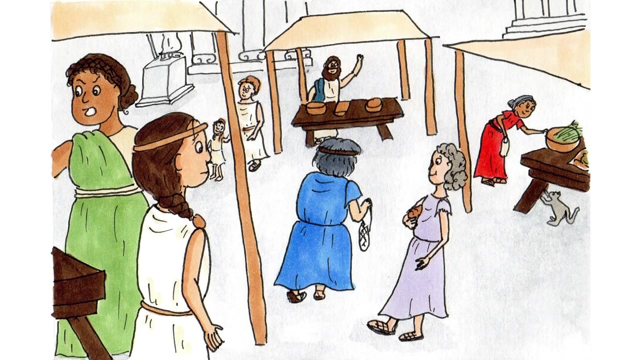 pause the video and tell someone what you think, or tell them why, or ask them what they think. As long as you're using your brain and having fun, you can't do it wrong. So let's get started. Delphi was shopping. This was a job that Delphi did not particularly enjoy. She looked around, 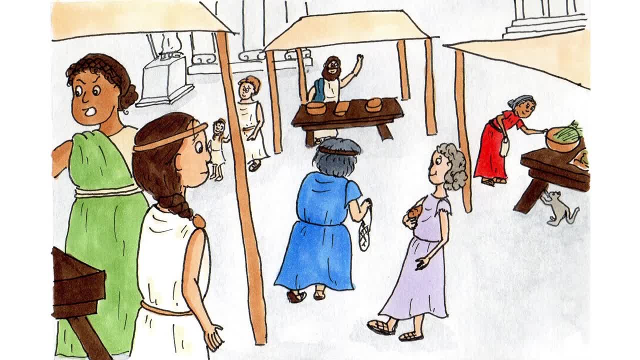 desperately at the emptying stores, trying not to be pushed aside by other women who were keen to get ahead of her. She was looking for an offering. This was one of the tasks that was often given to women in Athens. The city was a very religious place and believed in a whole avalanche of gods. 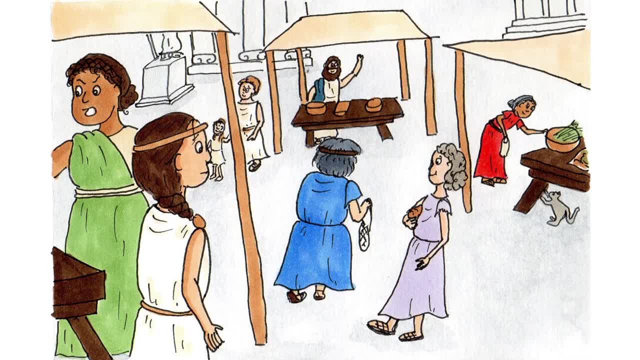 all of whom demanded their own festivals, sacrifices, rituals and presents On festival days, which felt like almost all of them. Delphi was often sent to buy something in the market that the god or goddess might find pleasing, and then take it to their 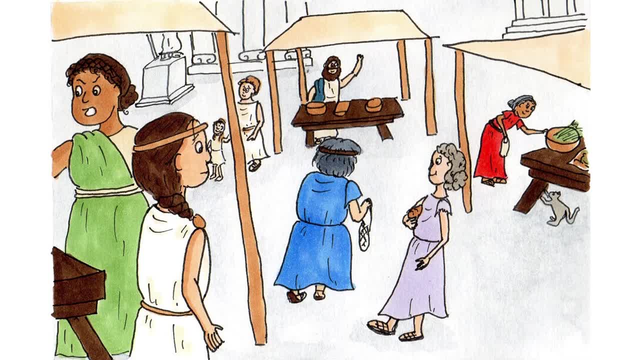 temple. She would then offer it up at the altar, say a prayer or mumble something convincingly, and then leave it for the gods. Nobody ever wondered what happened to it. next, Athens believed in its gods, Not for the first time. Delphi cursed her lack of money. 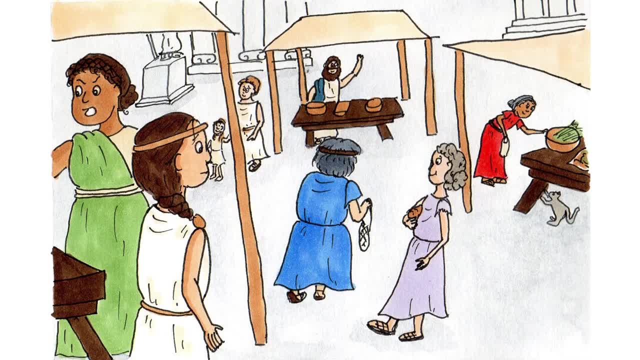 It wasn't her father's fault. He was a hard-working sculptor but it didn't bring in a lot of money and Delphi had no brothers to help And of course Delphi couldn't work. They weren't poor. 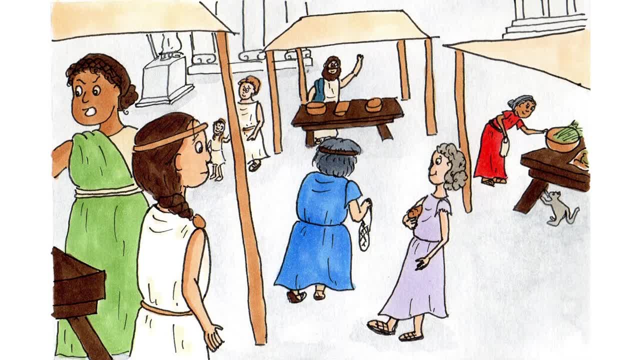 exactly. They just couldn't afford luxuries like good shoes or regular honey, cakes or offerings at festivals that weren't embarrassing. Delphi often wondered if the gods had noticed, but no thunderbolts had splattered her yet, so she supposed the gods weren't too angry at her. 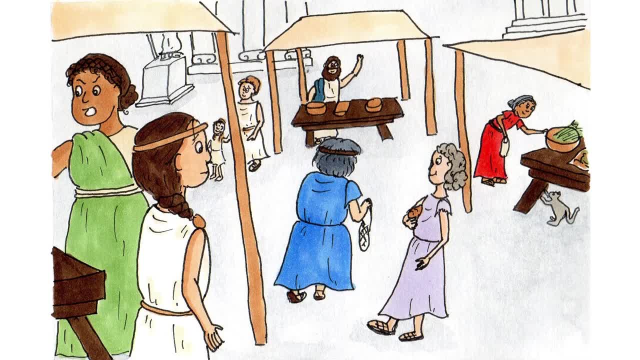 If only she had real money, She would enjoy shopping. then Think of all the things she could buy: 5., 6., 7., 8., 9., 10., 11., 12., 13., 14.. 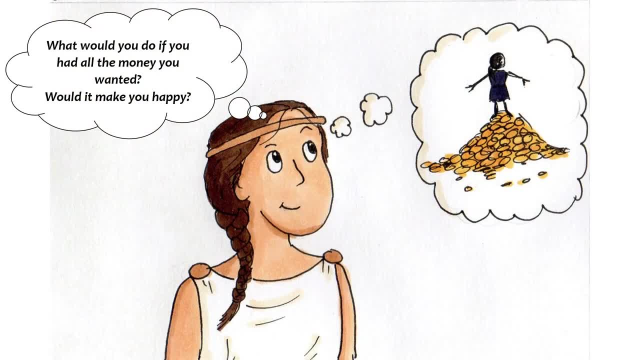 15. 15., 16., 16., 17., 17., 18., 18., 19., 19., 20., 21. 22.. But it'd make you happy. Delphi daydreamed for a while and had got through quite a big list of the things she would buy. 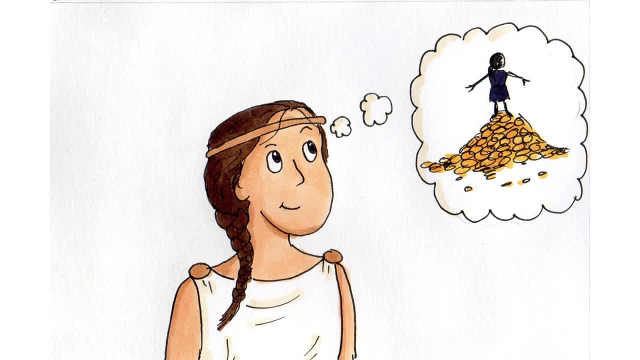 before her mind drifted back to Socrates. If she was rich, she could probably buy his freedom. It seemed to work like that. She could just pay everyone until they all agreed to let him go and forget all about it. Being rich probably made you a good person too, she considered You'd never need. 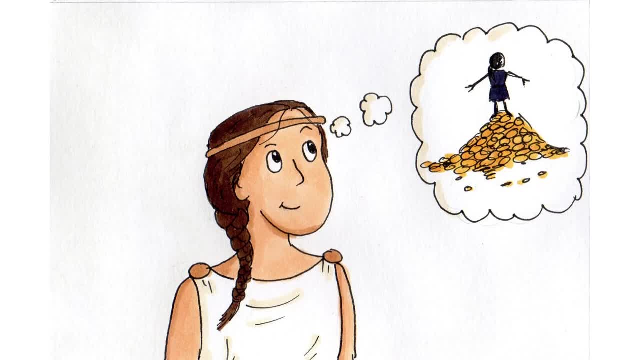 to do anything bad after all, because you'd already have a good person be able to get everything you wanted. Delphi sighed Asking what if was all very well, but it didn't put any more silver in her hand. After a bit more wandering around, she ended up buying. 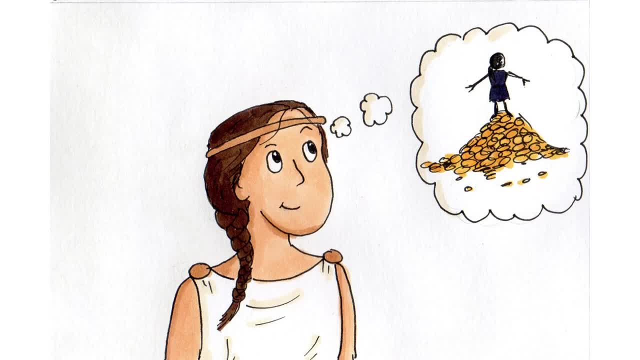 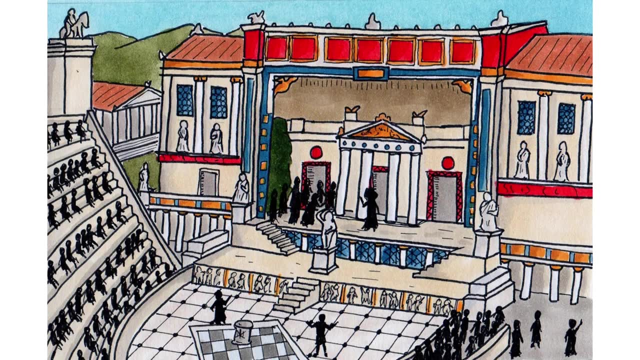 a small honey cake in the hope that the gods liked it as much as she did. With her little sweet-smelling package in her arms, she started to walk towards the edge of the agora, towards the theatre of Dionysus. Dionysus was the ever-popular god of wine, and today was one of 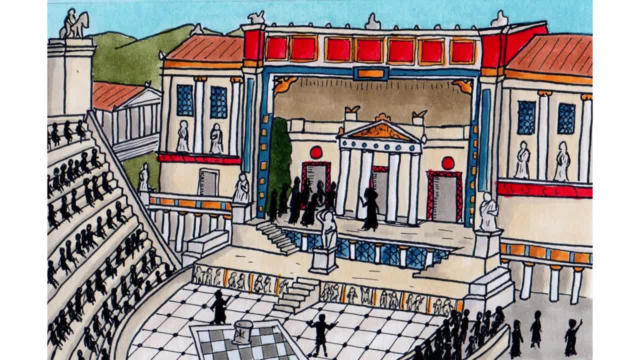 his many festivals. Athenians had taken to Dionysus in a very big way, ever since they'd realised they could drink as much wine as they liked, and because it was religion that made it okay. His temple was part of the huge theatre that dominated one side of the Acropolis Hill. 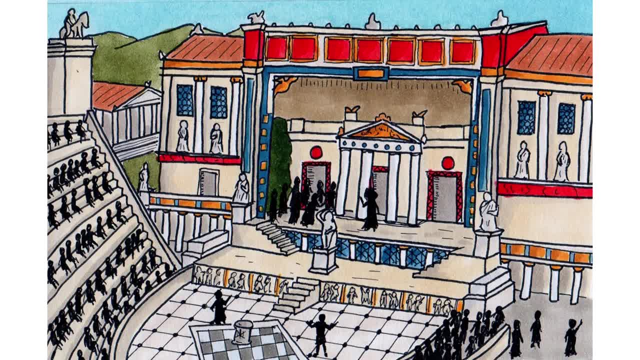 She hung back and waited until the last few women and the other young girls like herself had entered the shrine to make their offerings. When she was sure that she and a little package of cake wouldn't be seen, she padded forward on her bare feet and entered the shrine. 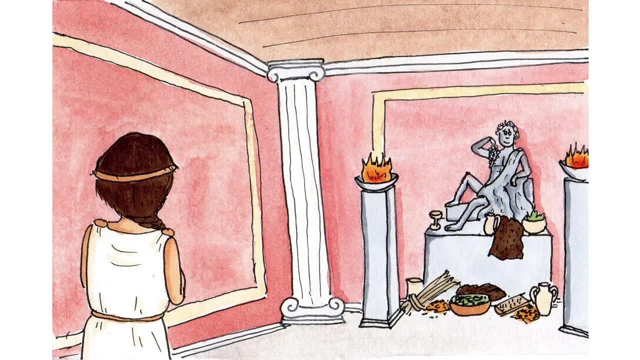 She had prepared herself for the sight inside, but it still stung. At the far end, lit by two flickering torches, was the majestic statue of the god himself, curly-haired, bare-chested and dangling a few bunches of grapes over himself, But it was the offerings that surrounded 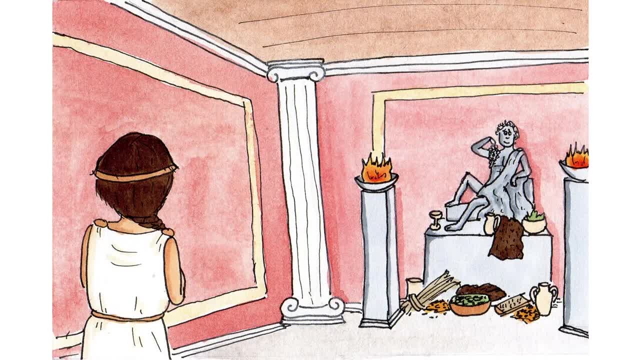 him which made Delphi feel sick: Oceans of wines, mountains of crops and fruits, hundreds of coins worth of oil and silver, gold and furs. it was everything she would never have. Delphi tried not to look at it, but the jealousy was almost overwhelming, Keeping her eyes to the floor. 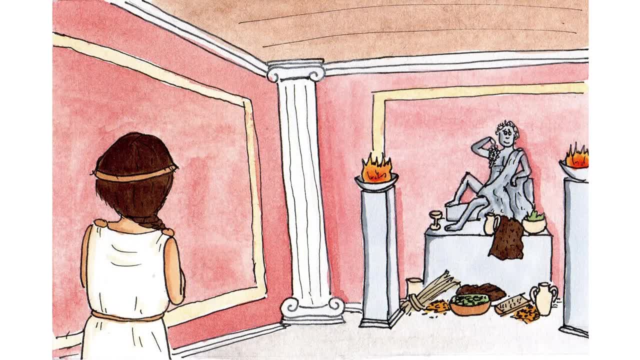 not looking at the statue's face. she brought her little packet of honey-cake to the feet of the god Dionysus. "'Sorry, this is all we've got for now' she whispered, bowing low as she placed it next to the pile of riches. "'But we—I mean my father and me—praise you. 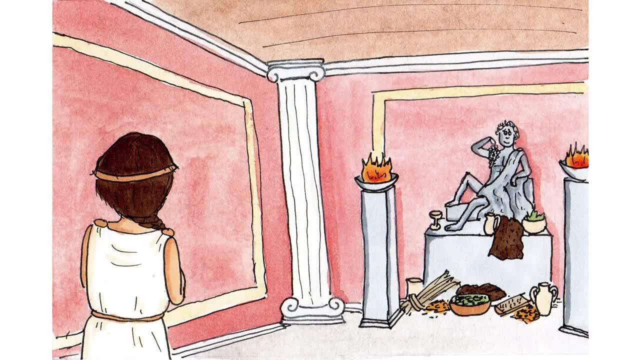 O mighty Dionysus, and offer you this gift of—honey-cake. It isn't enough for you, I know, but I ask for your blessings anyway'. Delphi paused for a few seconds. "'There's probably other things I'm supposed to say to you, but I'm not sure what they are'. 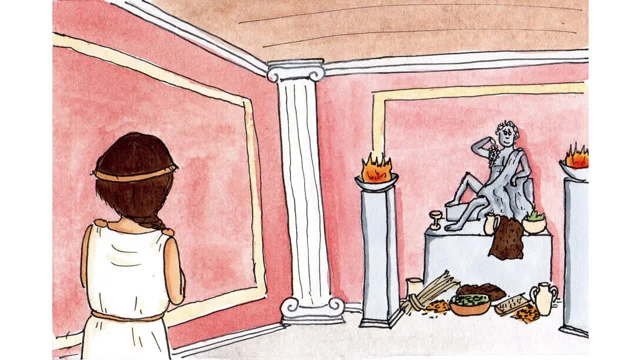 Delphi thought this probably wasn't a very good prayer, so she tried singing a hymn, but gave up on the second verse because she couldn't remember the words "'I hope that's okay, Um, thank you', Still keeping her gaze on the floor. 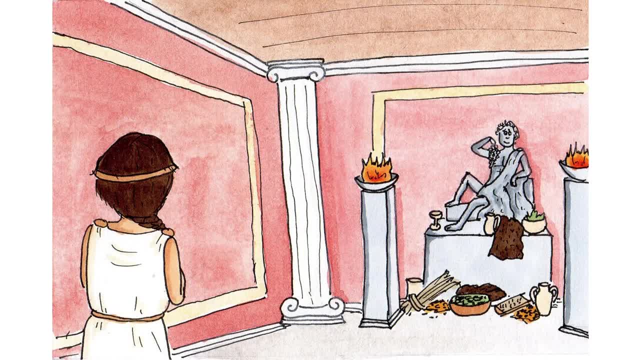 she slowly backed away and turned to leave. "'Why I haven't done anything' Delphi froze? The voice had sounded like two marble blocks being rubbed together and yet somehow also sounded light and cheerful, and it had come from right behind her. 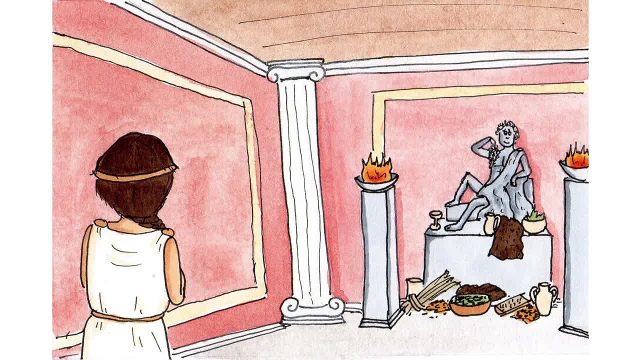 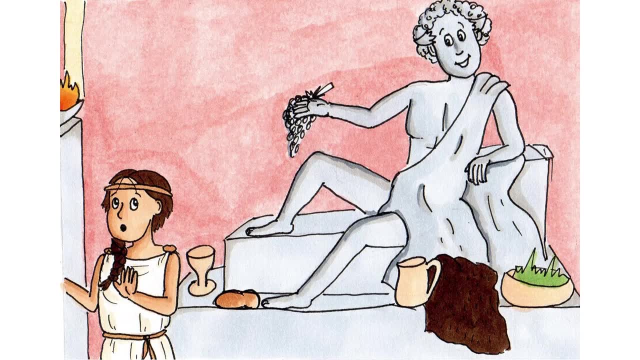 She turned around slowly, a deep horror rising up her chest. Dionysus smiled: "'What are you thanking me for? I didn't do anything for you, did I'. His voice was mumbling and slurred. He sounded like Delphi's father. 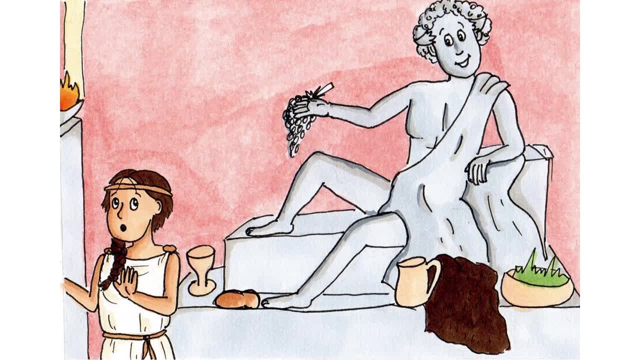 at the end of a particularly large drink of religion. The statue looked around and saw one of the big jars of wine at his feet. "'Ah'. He reached down and lifted it up to his lips, pouring a good amount of the dark red liquid down his throat in one go. 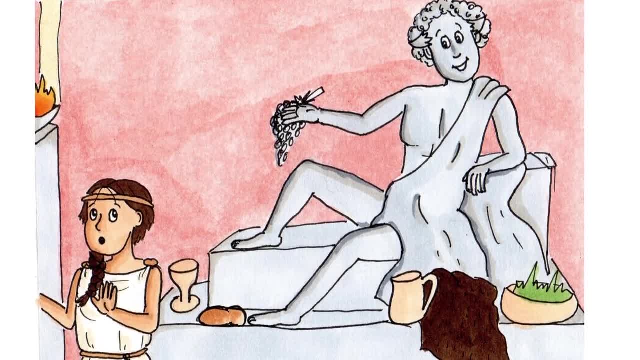 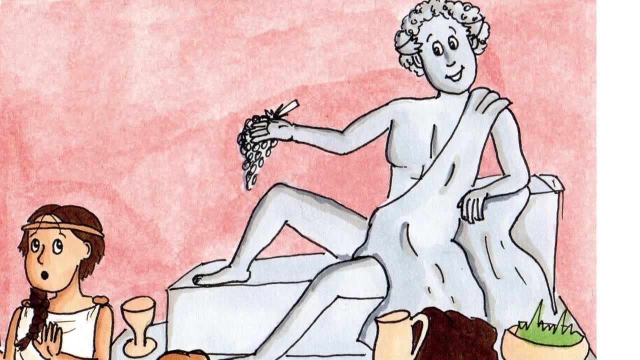 Delphi watched the statue's throat gulp. She couldn't move. "'Ah', sighed the god and burped loudly. He looked up again at Delphi, one eye slightly closed: "'Not sure who you are, to be honest, Was it—did you bring me'? 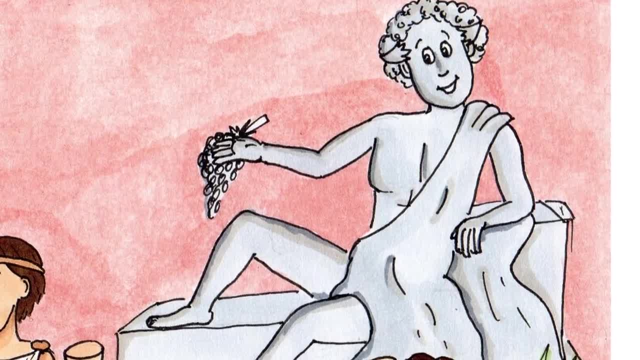 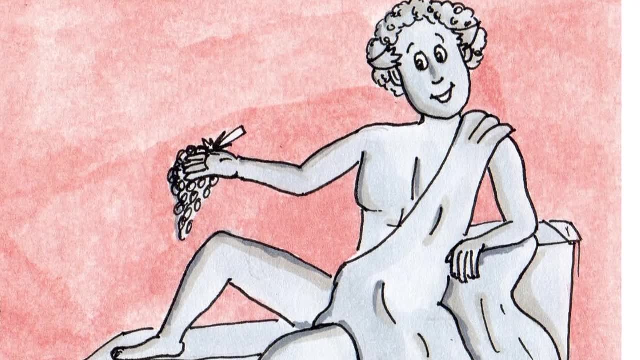 "'I didn't eat much of it. Please don't tell my dad'. Delphi blurted out. She had gone almost white with shock. "'Was it' mumbled, Dionysus? "'I didn't eat much of your honey cake. Just a corner bit broke off and I thought I—'. 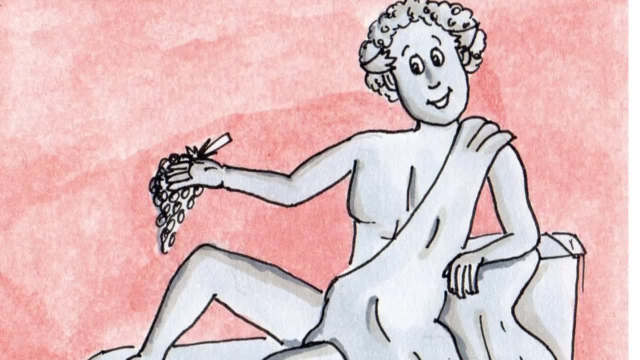 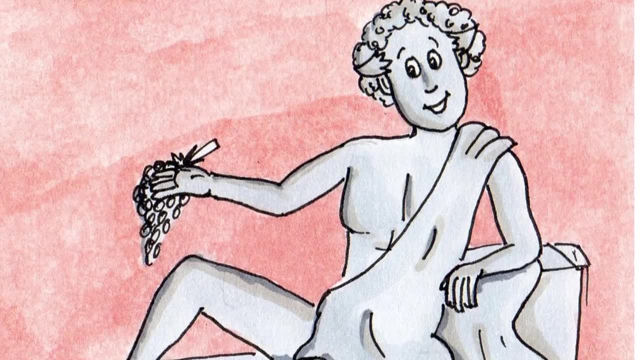 "'I didn't mind', he declared happily. "'You can have—have it all the rest of it if you like, Or would you prefer some oil to drink'. Delphi shook her head, her expression still frozen: "'You know—er—you know—you—'. 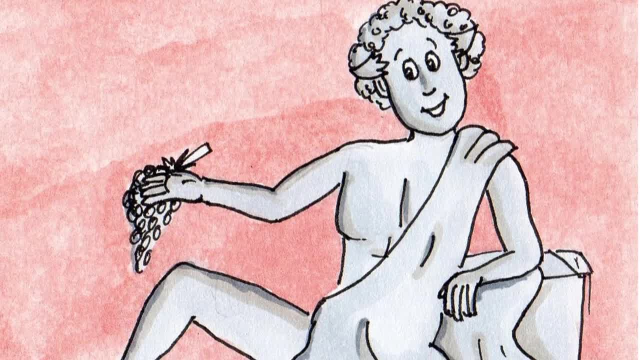 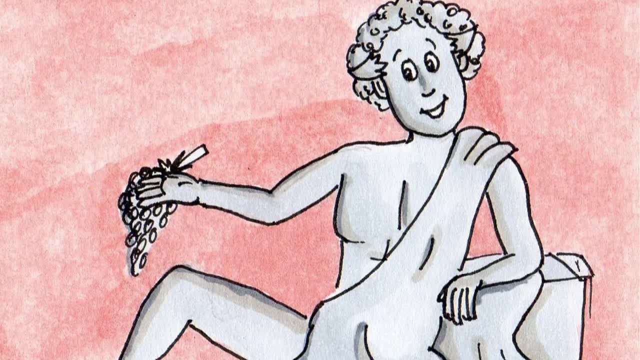 He waved his hands in a gentle direction. "'Do you know how many times somebody has said "'Thank you to me to-day'? Delphi shook her head again. "'They ask me for things you know. "'They ask me to make them happy or to kill their friends and save their foes, or something. 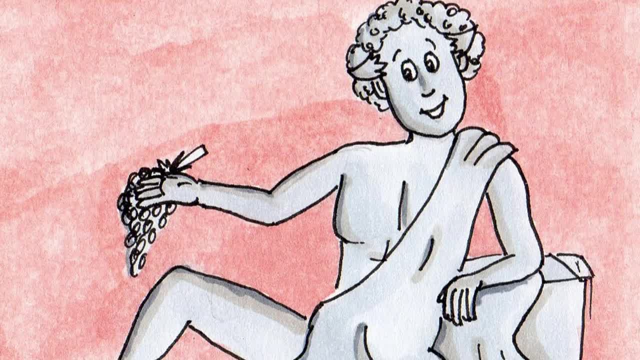 "'Not sure, Wasn't really listening, But they never—'. He stopped and held up a finger. "'Say thank you'. He looked thoughtful for a moment. "'At least—I don't think so. Perhaps I just missed that bit. 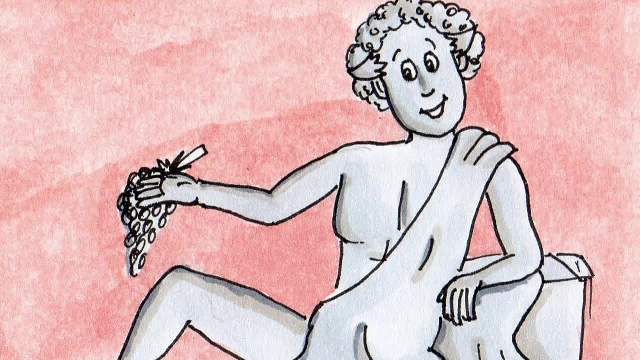 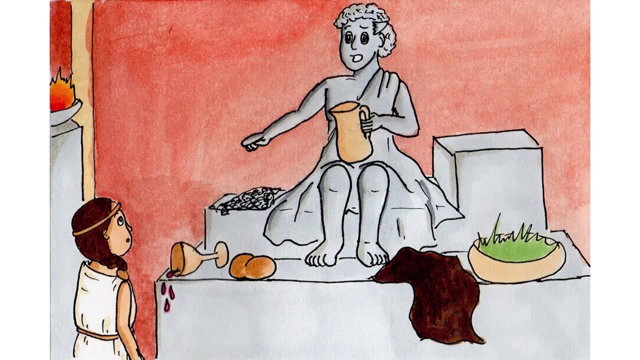 "'Hey wine' He picked up another jar and drained it in one go. Dionysus sat down heavily, sending a few more priceless jars rolling across the floor. "'So what would you like for your reward, then', He asked cheerily. 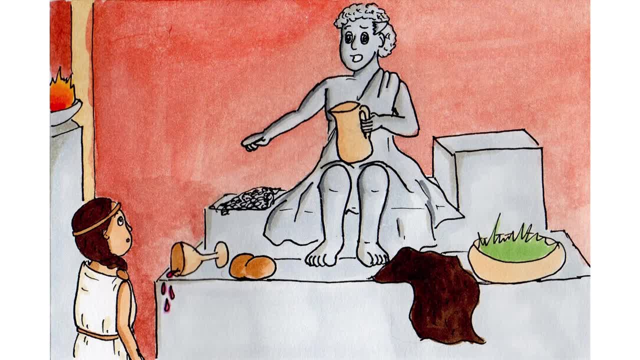 Delphi stopped bucking away. "'What I mean? what did you say? "'Oh mighty god of—' "'I said—' Dionysus cut in. "'What would you like? "'You brought me a nice present and sang a song. was it for me? 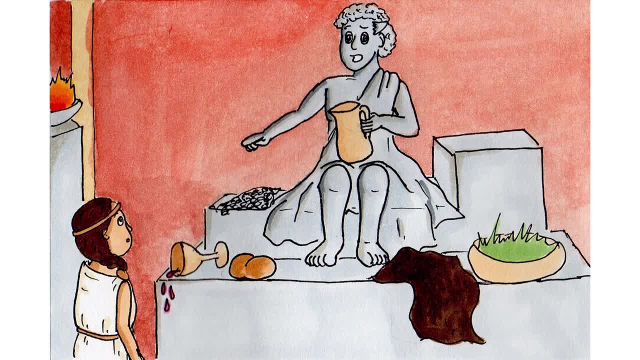 "'and now I'm going to reward you with something. "'cause that's what I do'. He thumped his chest proudly. "'Now anyway, so was it to be "'I—'. Delphi's jaw wobbled a bit. 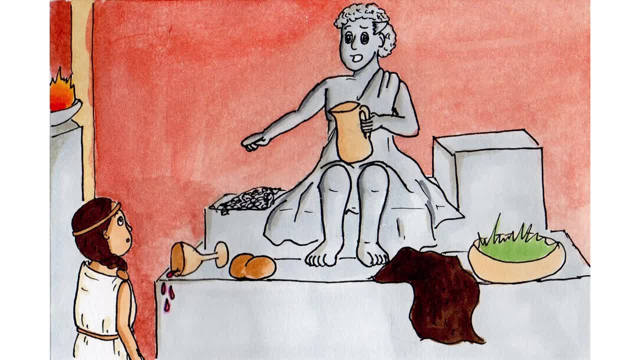 She wasn't quite convinced, but she really, really wanted to be. "'What kind of thing do you mean'? "'Gold' Dionysus declared: "'That's a good gift. I can do gold' "'Gold' Delphi's heart was starting to beat faster and faster. 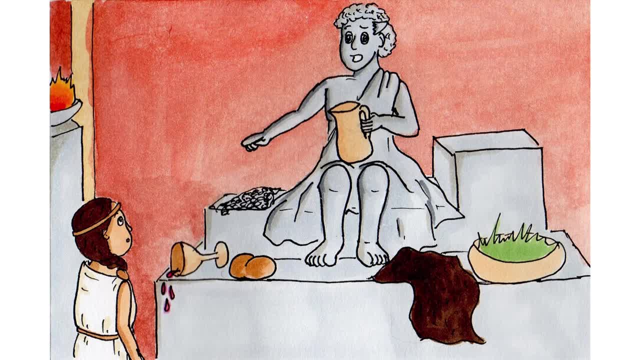 Was she dreaming? "'Gold, I can make you very, very gold—rich'. His eyes crossed for a split second and then focused on her again. "'Come on How much gold, Say it, I command you'. "'Commands from gods are usually very impressive things. 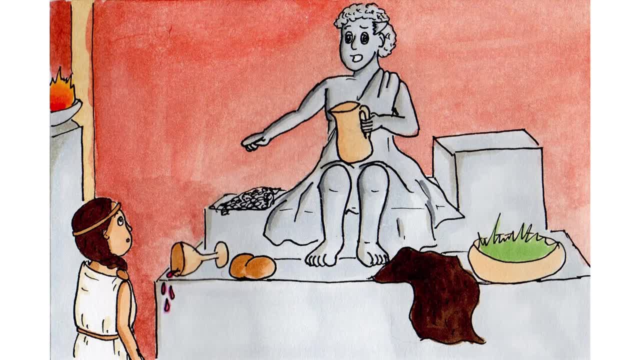 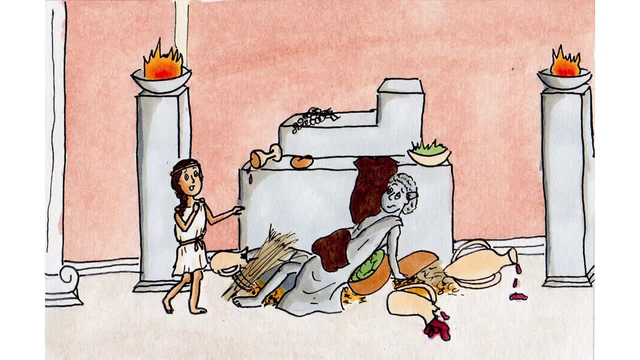 "'but Dionysus suddenly fell off the chest he'd been sitting on, "'and got his foot wedged in a particularly heavy-looking jug. "'Most of the remaining unbroken offerings fell onto his head. "'Ow' "'Um, are you okay', Delphi asked, stepping forward. 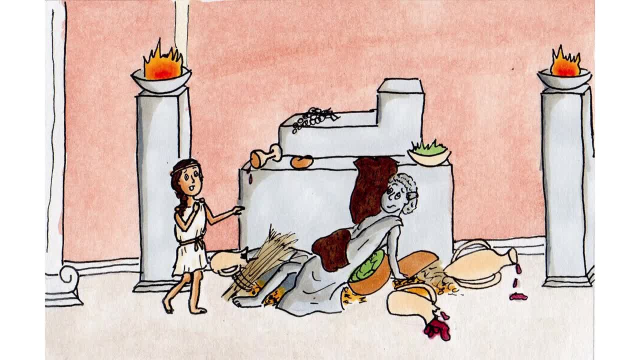 "'She realised that it may be worth getting a request in. "'before he passed out completely. "'Yes'. Dionysus appeared again out of the soggy furs, pulling himself up. "'Nothing a good sculptor can't fix. "'Now where am I'? 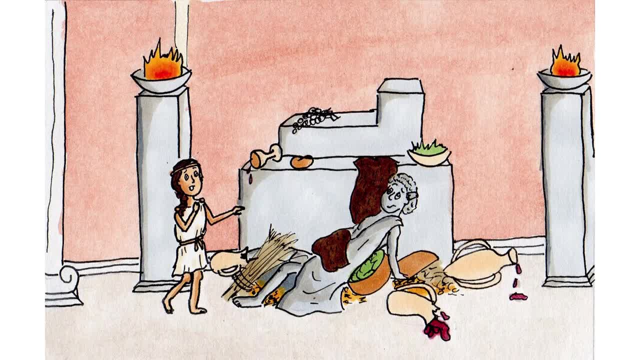 "'I will' "'Wish' Delphi started quickly before it was too late. "'No point in wishing small. "'Oh yeah, go on, How much gold'. Delphi thought quickly and greedily. "'Perhaps if her day had been easier or if she hadn't been panicked? 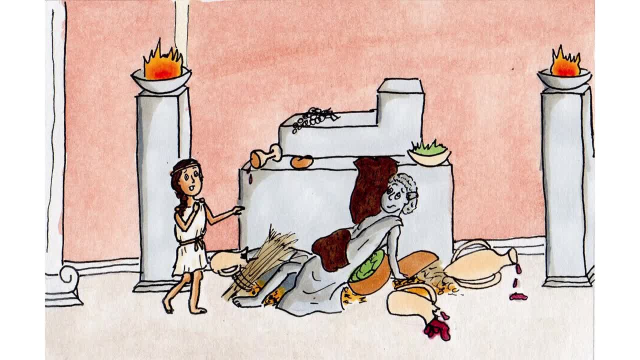 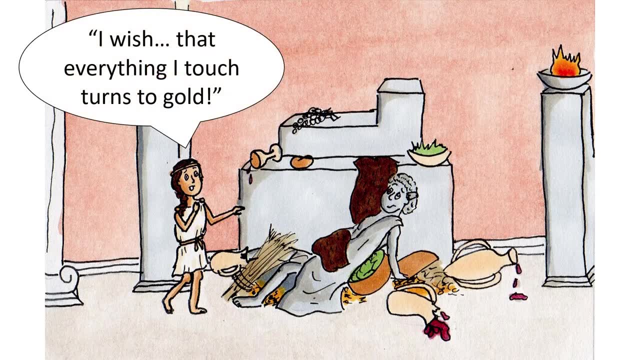 "'she might have thought carefully too' She whispered, shaking a little. "'I wish that everything I touch turns to gold'. She held her breath and looked at the god who was nodding. "'You know what? That sounds familiar somehow'. 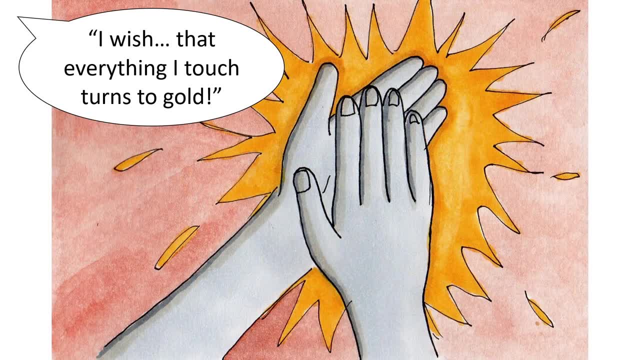 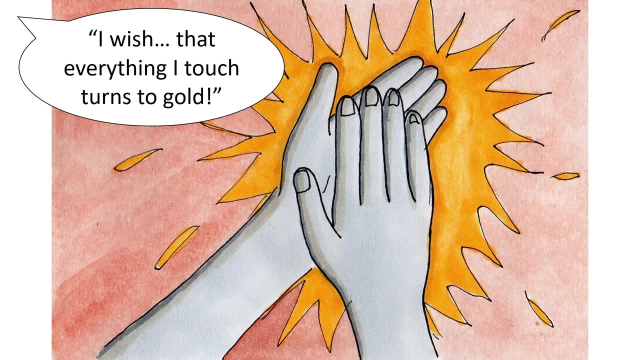 He shook his head: "'From somewhere'? "'From sunrise'. Dionysus brought his hands together in a clap so loud that it shook the universe. It went through Delphi like a thunderbolt. Later, all she could remember was the gleam of gold in her eyes. 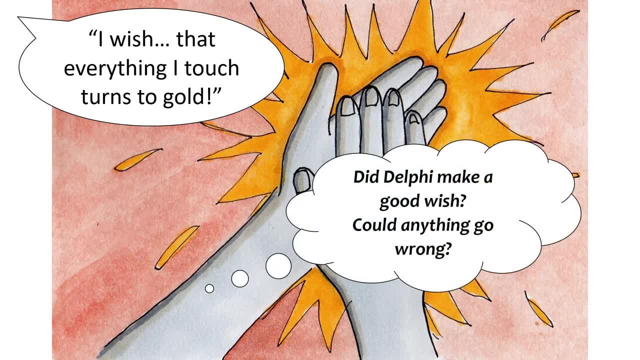 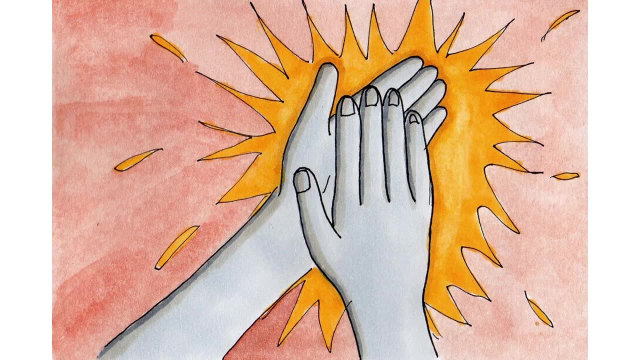 and the sound of laughter in her ears: "'Did Delphi make a good wish? "'Could anything go wrong'. Delphi woke in her own bed in her own house, when it was still dark outside. She rubbed her eyes and stretched her arms over her head. 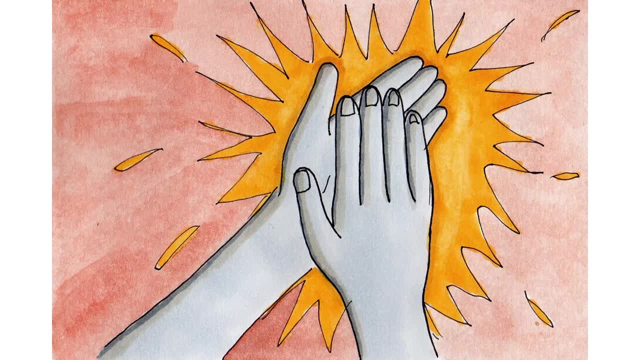 That had been a very strange dream. She groggily got to her feet. She felt like she had been awake all night as she had drunk some of the wine. Her memory of the previous evening was a little patchy. She remembered buying the honey cake and then levering it with all the other offerings. 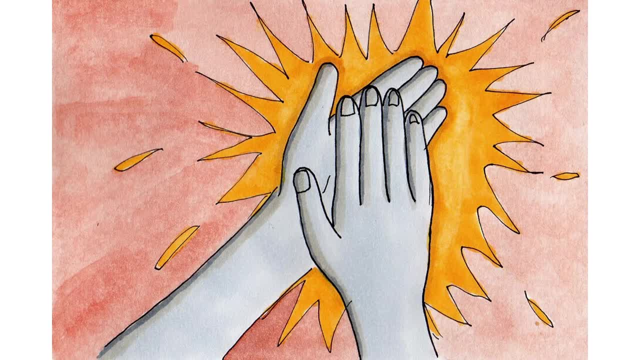 and then she had said a prayer, and as she tried to put her thoughts together, she stepped outside into the courtyard and looked at the sky. It was dawn, but even as she watched the sky was brightening, and she waited until the sky started glowing a deep dark. 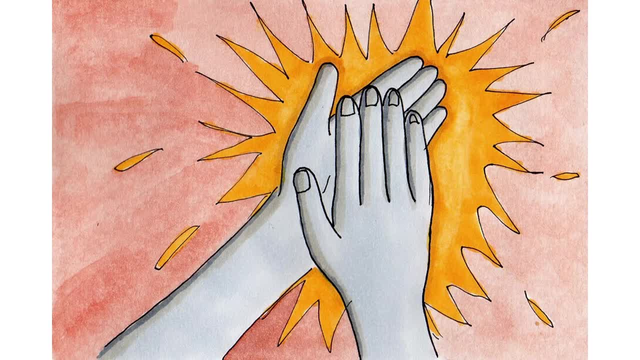 It was gold. Delphi suddenly held her breath: "'It couldn't be, could it' "'No, she must have been dreaming. She must have'. She laughed to herself For a split second there. she actually thought that—'. She looked down. 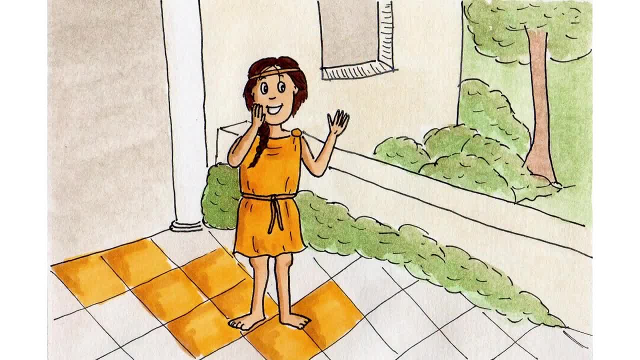 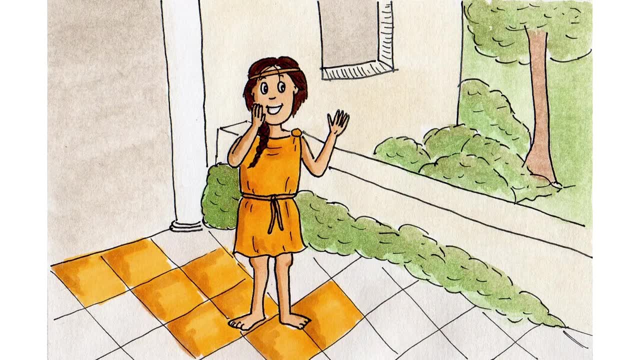 She was dressed in a tunic of shimmering gold. Delphi's mind exploded. She took a few deep breaths, trying not to be overwhelmed by a mix of sheer excitement, disbelief and panic. She looked at the floor Underneath her two bare feet. both the flagstones were shining a dull gold. 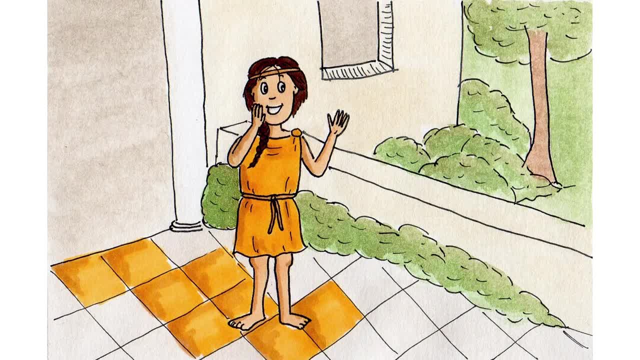 She stamped on one of them, She looked at the other, She looked at the other, She looked at the other one and it felt cold and real. Her wish had come true. Even her knickers had turned to gold. Her heart leapt. 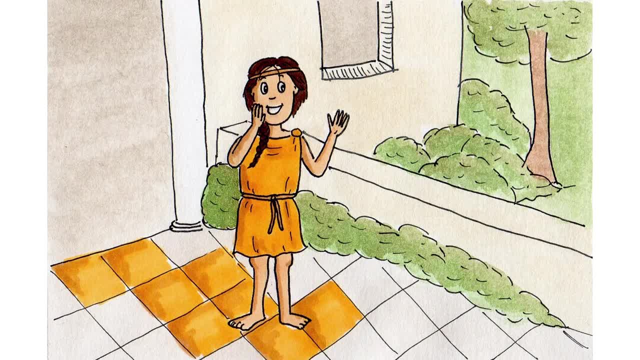 She was rich, They were rich. No more embarrassing offerings to the gods, No more saving up for small scraps of honey cake. She could get anything she wanted. Smiling like a lunatic, Delphi carefully stepped through the courtyard, delighting in turning each paving slab gold as she trod on it. 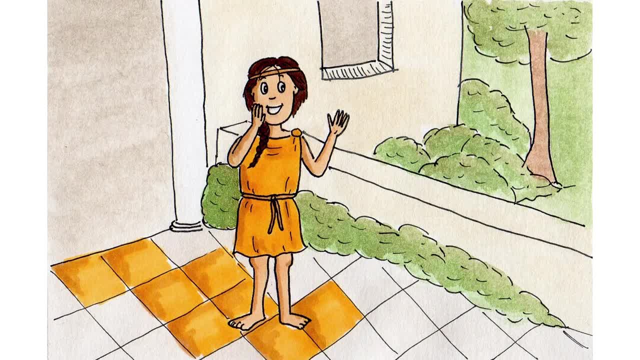 She was going to be famous. People would come from all over Greece to see her, the girl with the golden touch. She reached down to a delicate white rose which grew in the corner of her courtyard and gently poked it with her finger. 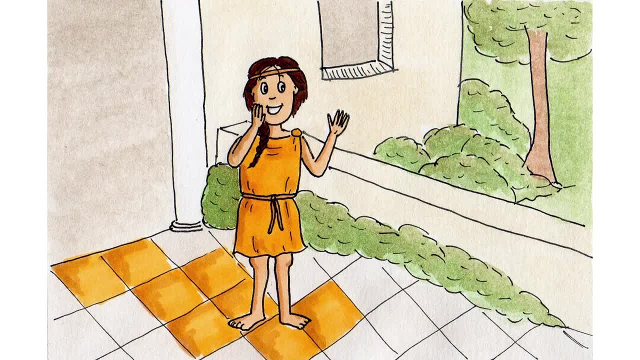 It instantly turned golden, its delicate petals catching the early glow of the sun. Right, she thought, Quick breakfast, then she'd wake up her father. What on earth was he going to say? She skipped back towards the kitchen and spotted some apples on a wooden plate. 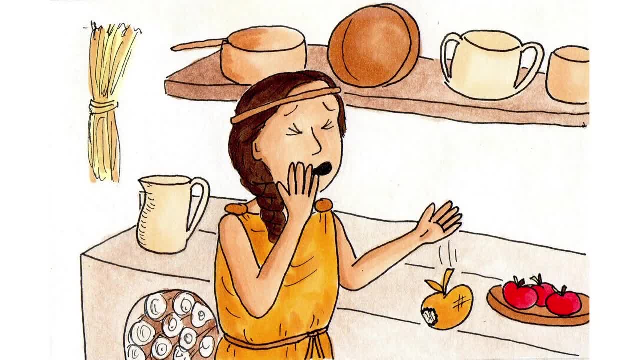 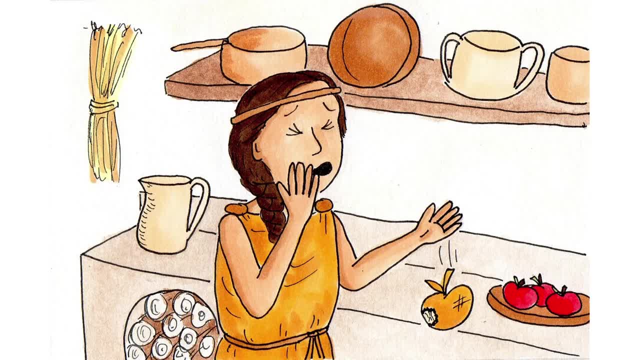 She tried picking up another apple with a bit of cloth. The cloth turned gold, but the apple didn't. But as soon as her teeth touched the skin, Ow, she cried again, holding her aching mouth. It is a credit to her that she didn't panic then either. 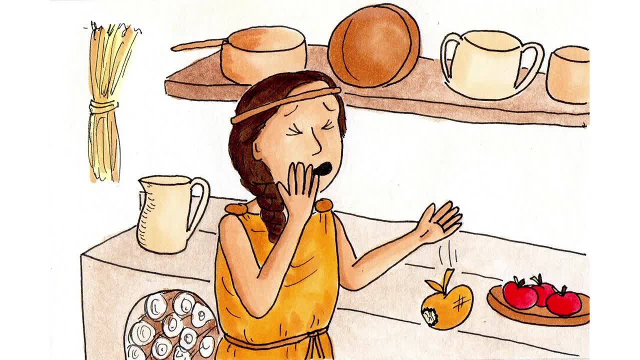 deciding that she would worry about it later. As long as she could have a drink, it would be all right. She poured some water from a golden jug into a golden cup and brought the water to her lips. She almost choked. She dropped the cup where the remaining water had turned solid. 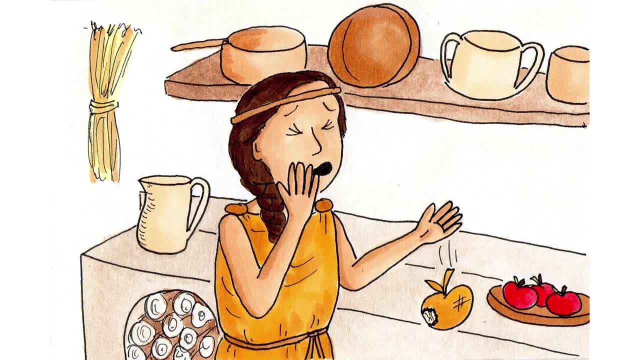 She reached into her mouth and pulled out a clump of gold. She threw it on the floor. She would have panicked then, but she heard footsteps behind her, so she whirled round and flew forwards. Dad, I've done something really stu—. 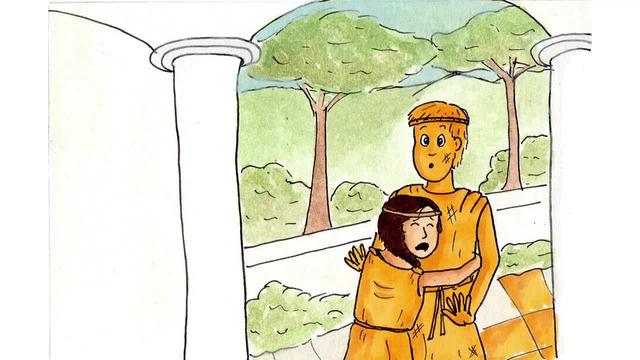 She ran into his chest. Where her father had been entering the courtyard, there was now a full-size golden statue of her father. He had often joked that after a lifetime of making statues for other people, one day he'd have a statue of his own. 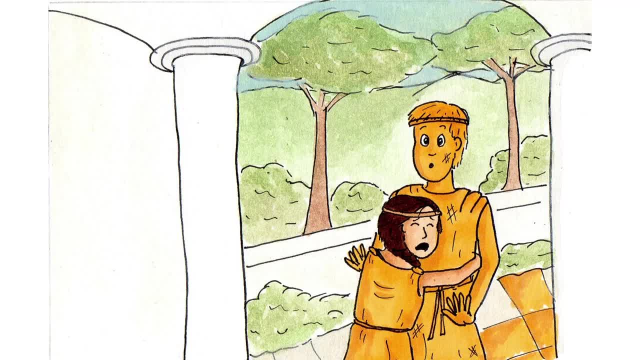 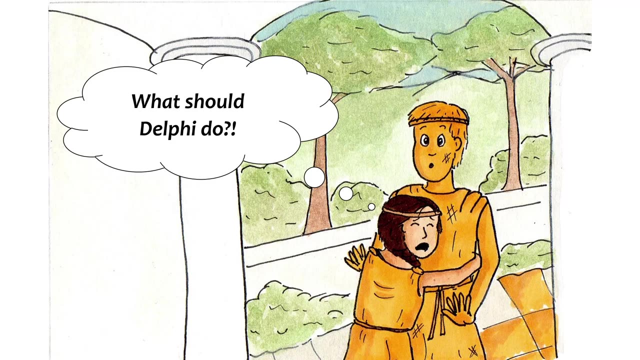 He had no idea that the day would come so soon. Delphi looked up in horror at the golden gaze of her father and blinking and cold. Then she panicked. What should Delphi do? Dionysus Delphi skidded into the shrine. 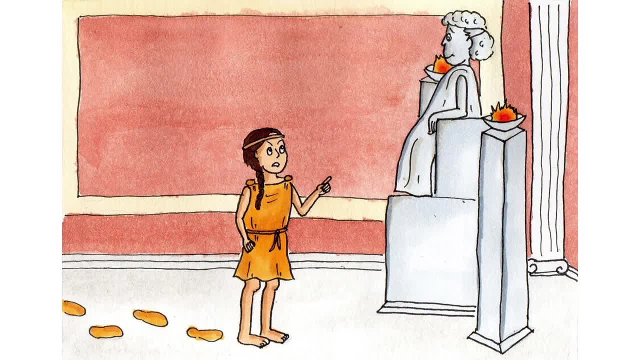 Her bare feet had left a trail of golden footprints from her house all the way here. Her eyes were red, but she hadn't been crying. If she'd cried, then she might have given up, So she had got angry instead. She stuck up her chin in the direction of the statue, which stood cold and still. 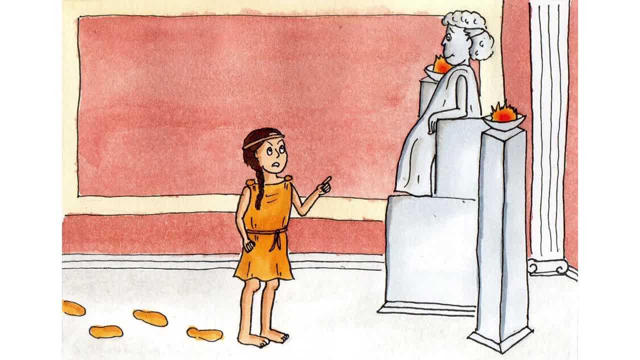 Her hand shaking a little, she started to reach out towards the statue with one outstretched finger. Would you like it if you were turned to gold forever and ever? The statue suddenly flinched and backed away from her stone muscles grinding against each other. 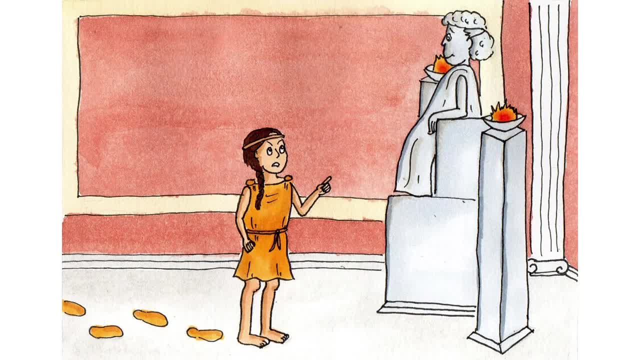 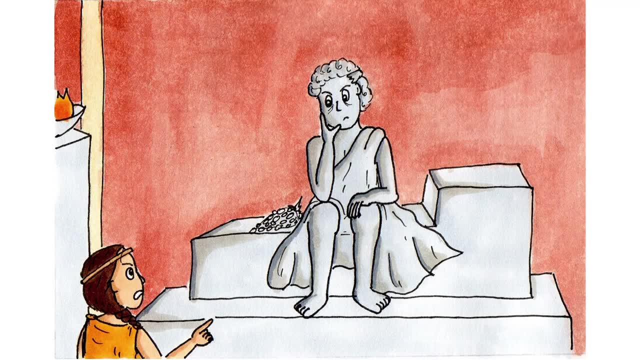 Ah, Please don't. Delphi lowered her finger. You tricked me. You knew I was wishing for something stupid and you let me do it anyway. Ugh, Not so loud. Dionysus protested feebly, holding his hands over his delicately carved ears. 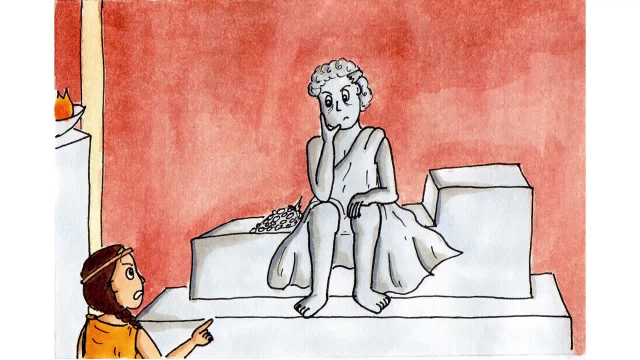 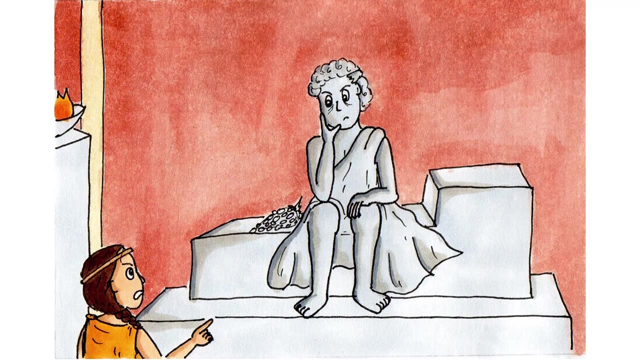 He sounded a lot more fragile this morning. What, what time is it? Sunrise, snapped Delphi, Did you realise? your present meant I couldn't eat or drink or anything. Ugh, Dionysus moaned and sat heavily down on his stone pedestal, holding his head in his hands. 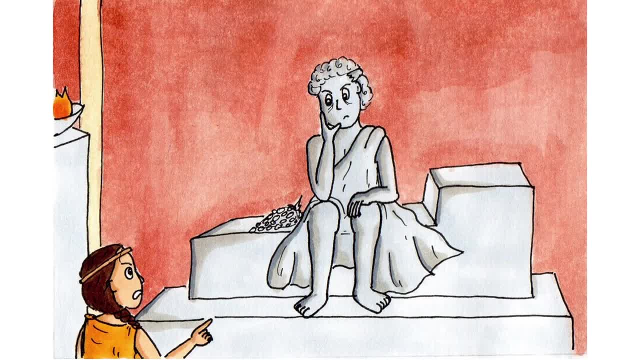 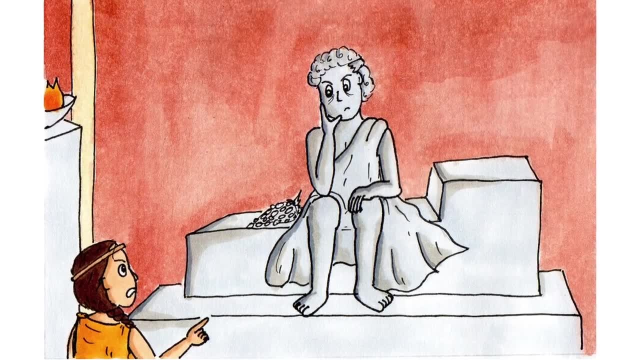 Why are you back here? It's the morning after my festival. I was planning on sleeping for a week or two, Never mind that This is all your fault. Are you going to help me or not? Delphi demanded before remembering who she was talking to. 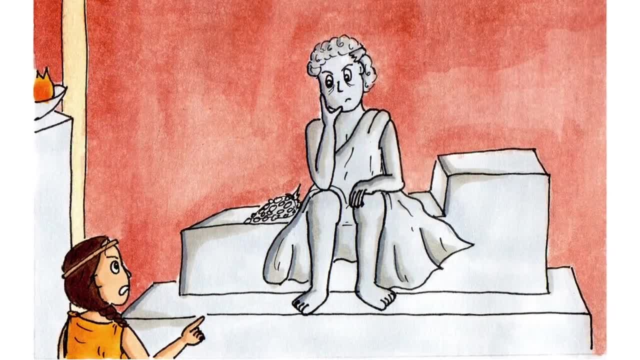 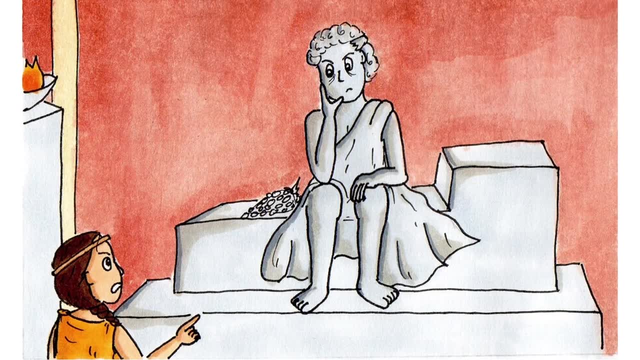 I mean Please, All right, all right. The statue took a few deep breaths. I don't know what you're complaining about. Perfectly good wish. There was this other bloke, Midas, I think his name was. 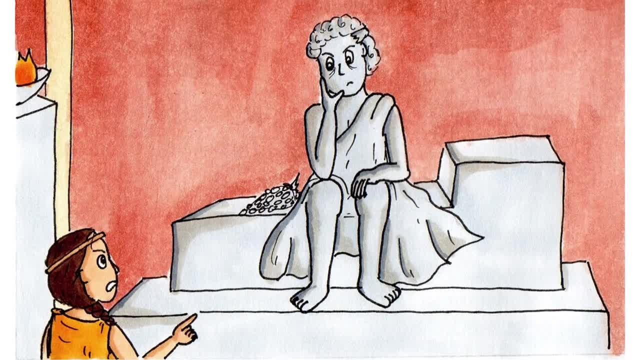 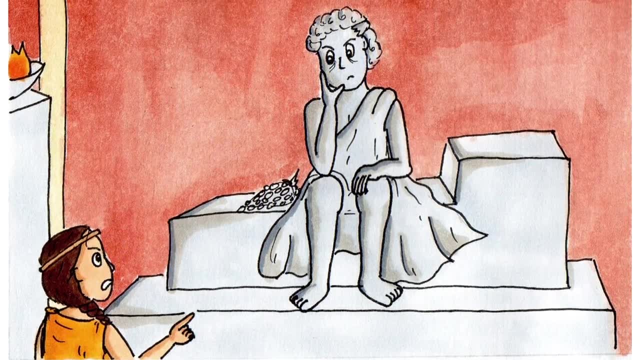 He wished for the same thing. you did Never heard him complaining about it. Dionysus thought for a moment. Or was he the bloke who wouldn't shut up about it? That's right, Midas, He was a whingy one actually. now I think about it. 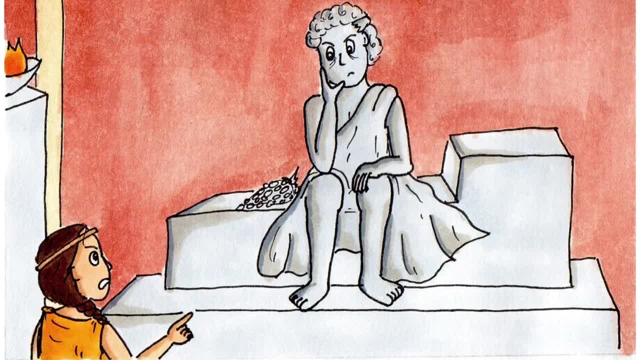 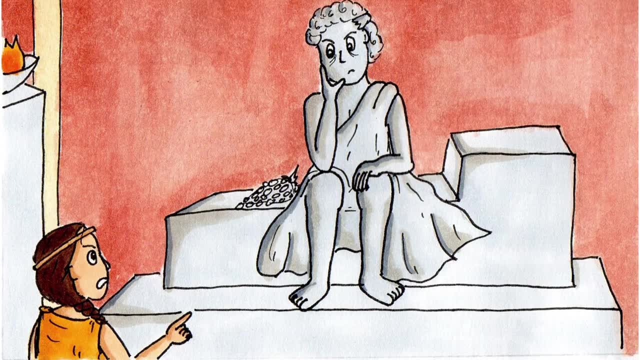 Hello, Delphi cut in impatiently. All right, okay. so What do you want to change your wish to? then Delphi was taken aback. Change my wish, She asked. You mean I can have another go? 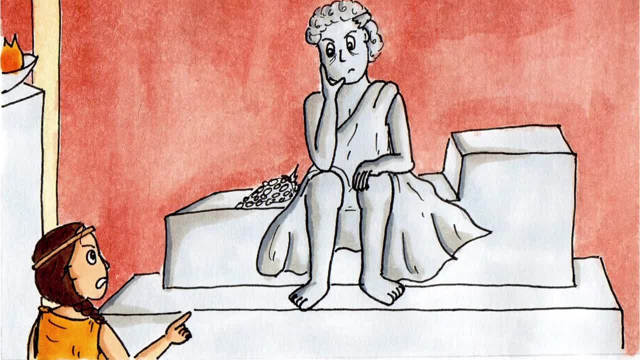 Will you turn all my stuff back to normal again? Oh, and my dad? She added as an afterthought: Listen, kid, I'll turn the whole damn world upside down if you'll just leave me with my headache in peace for a bit. 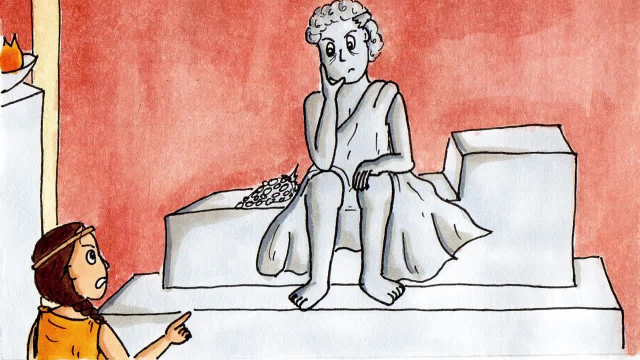 He moaned, rubbing his eyes. So I can still wish for gold just differently. Delphi asked This was going considerably better than she was expecting. Yeah, yeah, You can still turn to gold by touching it if you like. 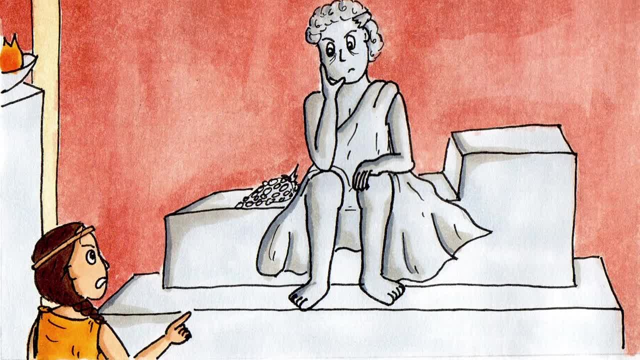 But I'm not undoing it again. I'm not some used chariot salesman. You leave me alone after this one. all right? Delphi shrugged. That seems fair. But a little doubt wormed its way into Delphi's brain. 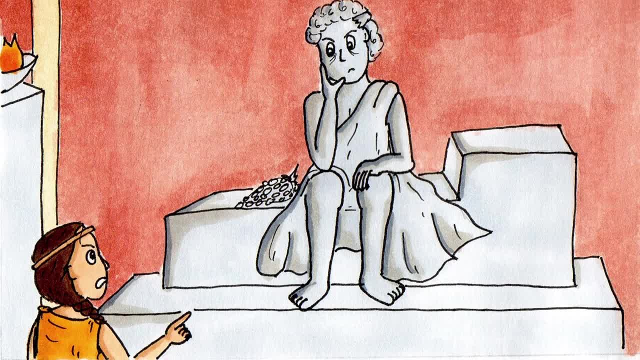 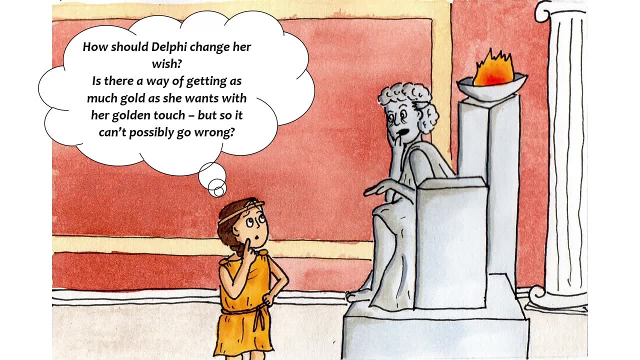 That means that whatever I wish for this time must be perfect, doesn't it? I mean, it can't go wrong this time, can it? How should Delphi change her wish? Is there a way of getting as much gold as she wants with her golden touch? but so it can't possibly go wrong. 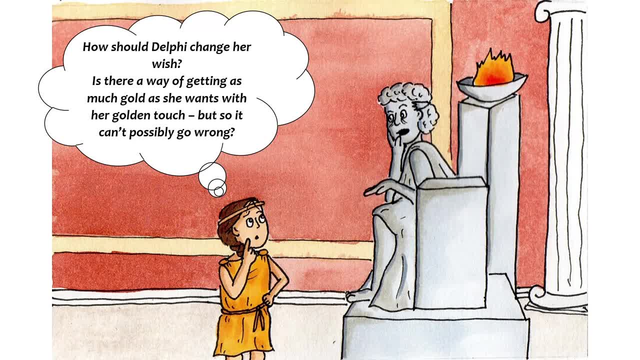 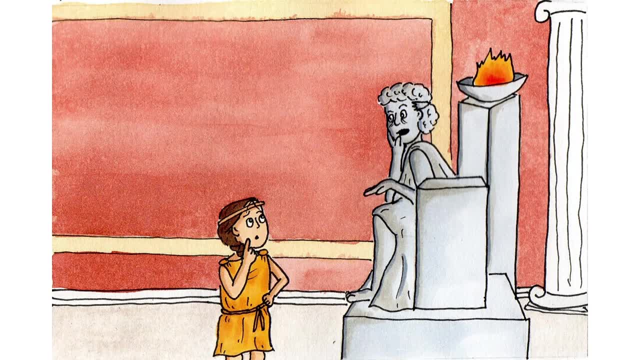 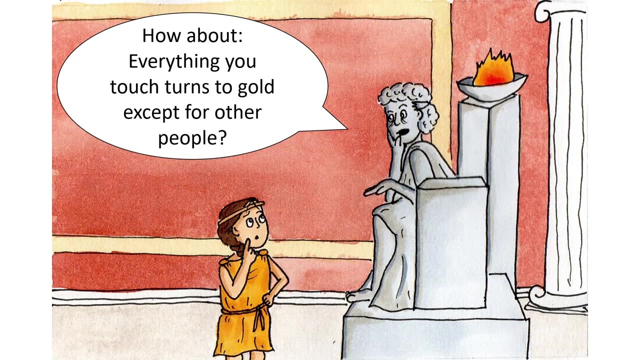 Delphi thought for some time She really did have to get this right. I don't know. she confessed. Look, how about everything you touch turns to gold, except for other people, since you seem to like them so much. Would this work? 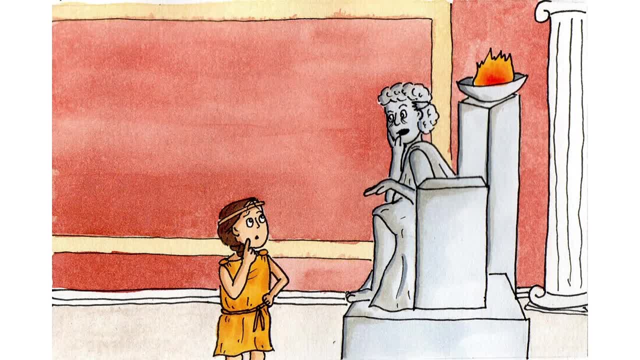 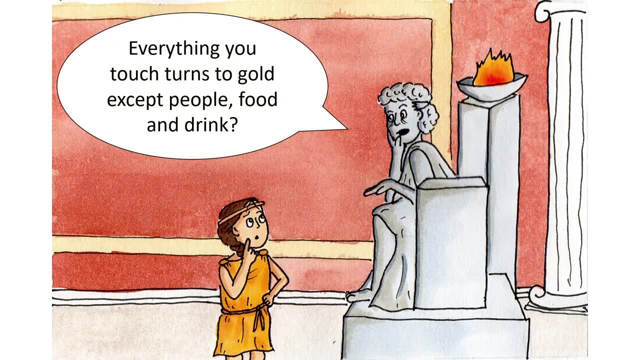 Delphi shook her head immediately. I'd still need to eat and drink, wouldn't I, She pointed out? Fine Dinosaur answered: How about everything you touch turns to gold, except people, food and wine? then I mean drink. 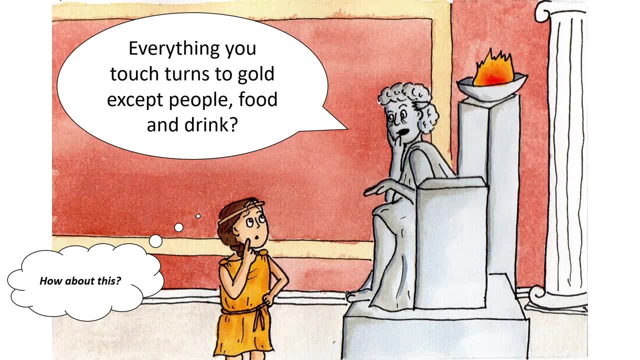 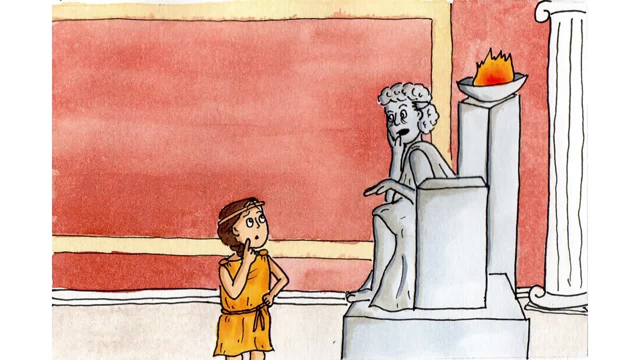 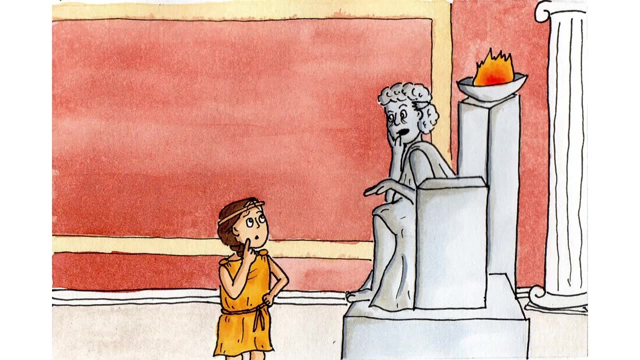 How about this? No, because what if I touched a book or something, Or firewood, Or my pet tortoise? I don't want those things to turn to gold. They're better as they are, aren't they? Her face was screwed up in concentration. 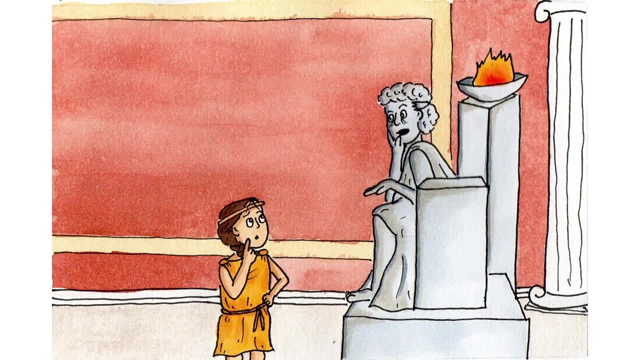 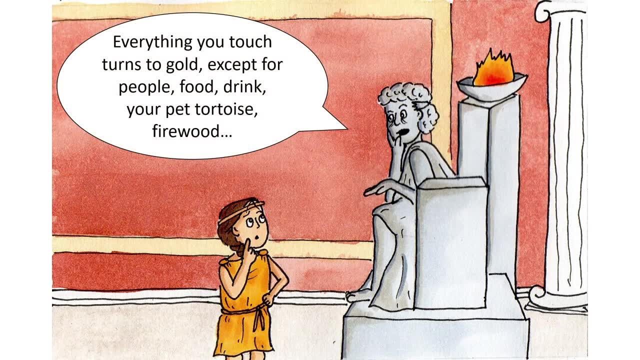 Dionysus, let out another theatrical sigh. Fine, How about everything you touch turns to gold, except for people, food, drink your pet tortoise firewood, was it? And erm, He trailed off. Is there a problem with a wish like this? 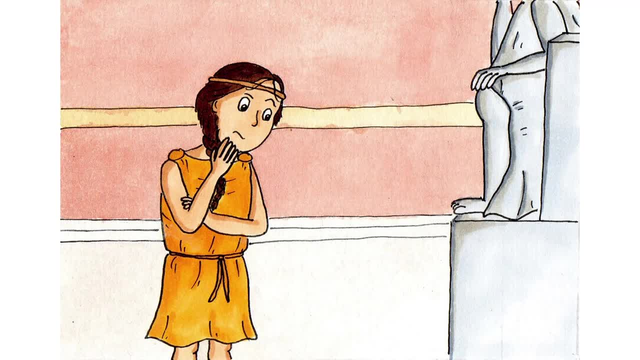 Delphi ground her teeth together in frustration. But it's not going to work, is it? There'll be loads of things I don't really want changing And I can't very well work out every single thing that I'm ever going to touch that I don't want. turning to gold, can I? 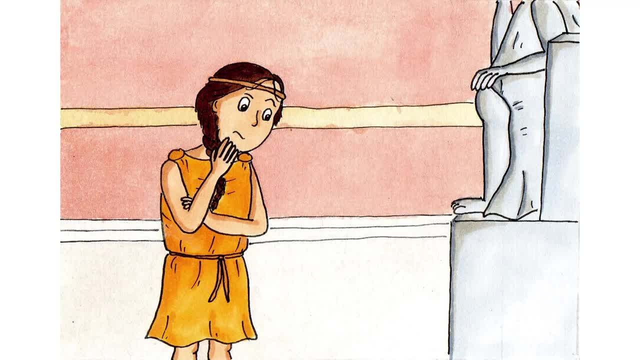 I mean, I'm bound to forget something, aren't I Don't look at me. It's your wish. Dionysus pointed out. Look, can't you help? She asked him irritably. This is hard. Oh, I don't know. 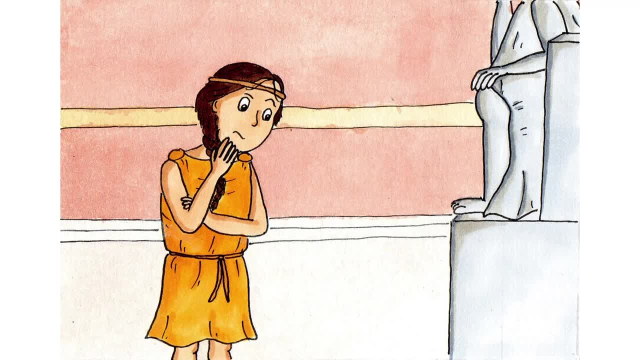 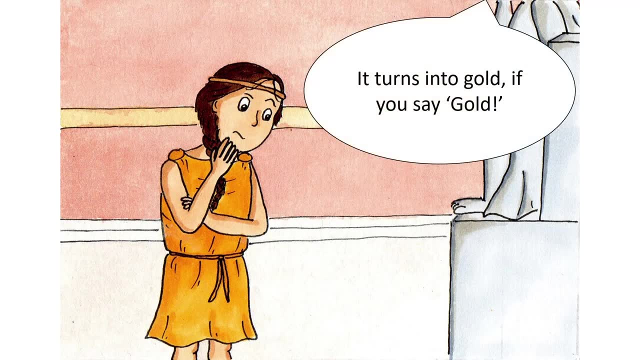 I don't usually think of wishes, I just find them funny when they go wrong. He started to laugh, but immediately winced and stopped holding his head again. How about it turns into gold? if you say gold, Is there a situation where this could go wrong? 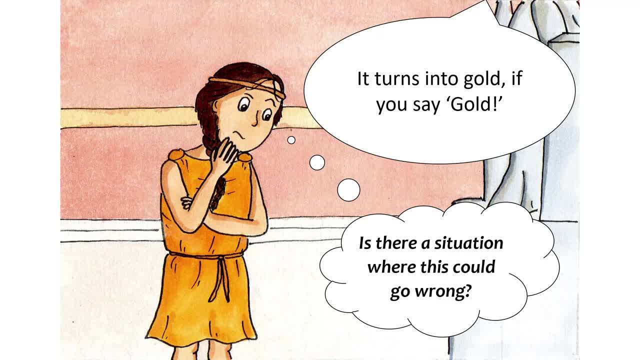 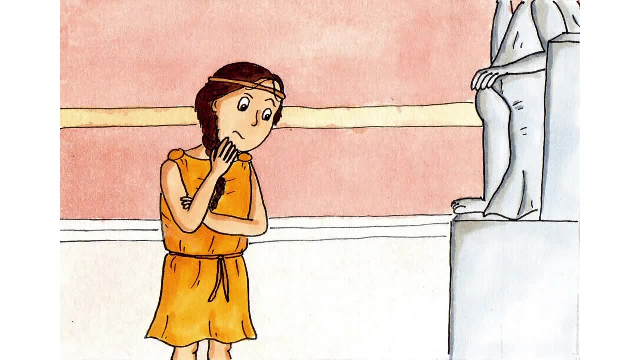 Delphi thought for a moment, then shook her head. What if I was holding hands with my dad and then I said something like Look at that girl's gold necklace? Then he'd still get turned to gold again, wouldn't he? 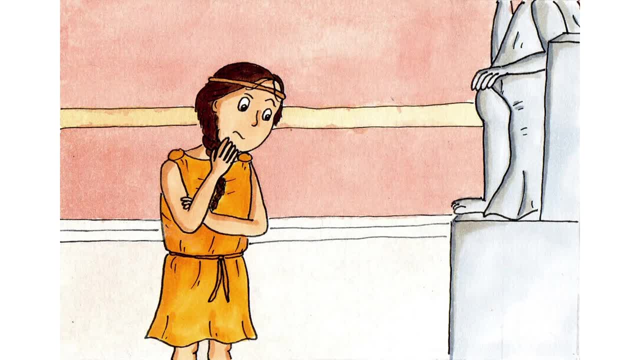 Dionysus nodded glumly: Oh, wouldn't it be easier just to have a golden father? I mean, it would save a lot of—. No, They both went silent. Delphi was thinking and thinking, But she just couldn't think of a situation where it didn't work. 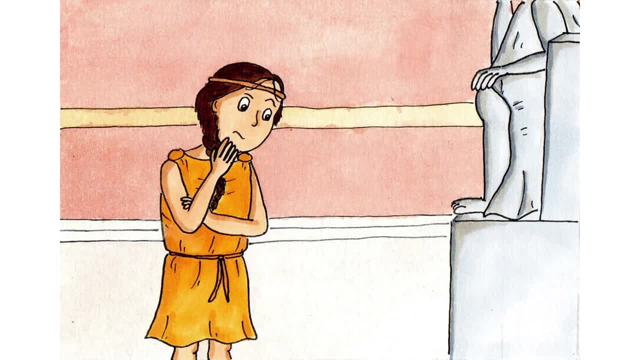 What if it spiralled through her brain like tornadoes? How about we lose the golden touch thing She suggested? That just seems silly. Can't you just give me some gold? All right, How much would you—? No wait, I'd just run out, wouldn't I? 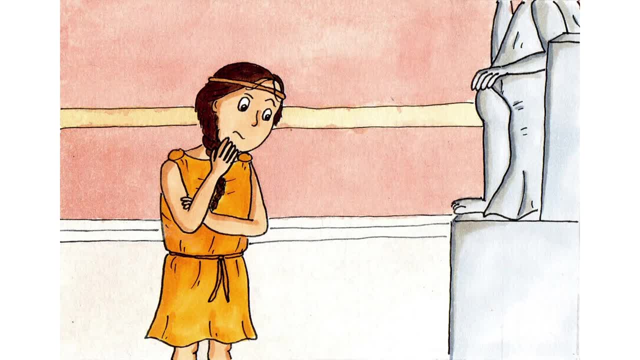 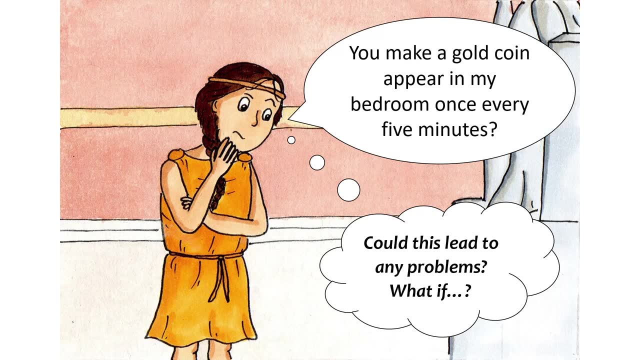 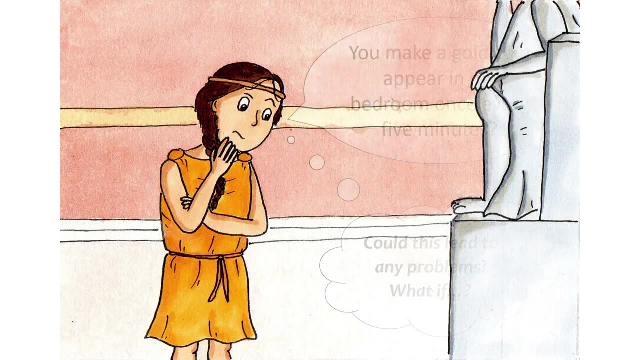 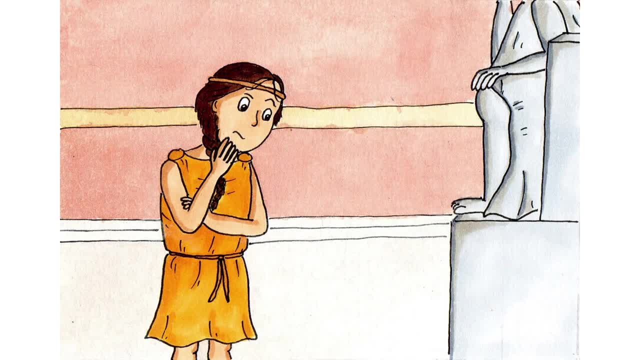 It seems like a lot of work, though. Do you realize? I'd have to make two thousand and sixteen gold coins every week, WOULD YOU said? Delphi slightly impressed at his math skills, But if it will get you to leave me alone—. 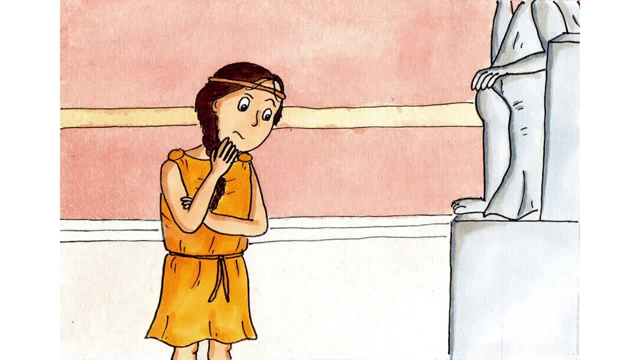 CHAPTER IV. No wait, Where would put them? I mean, my room's not very big. if it went away for a few days you could just come and steal them all, And if it went away for longer I'd probably drown in them. 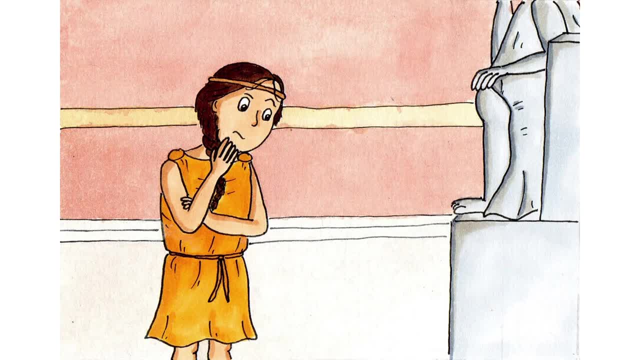 QUICKLY TH安. And you thought, Ytter, And what if I move house? DIONYSUS ACTIONS almost collapsed. Oh and hang on a minute. Delphi held her finger up, her thoughts now dancing. Even if I did have loads of gold, then people would know, wouldn't they? 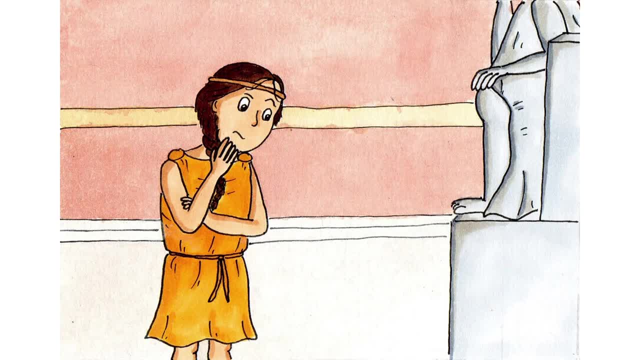 They'd want to know where I got it from, and I wouldn't be able to stop them taking it from me. so it'll just mean everyone's got lots of gold. Then what's the point? Gold's only special because nobody's got much of it. 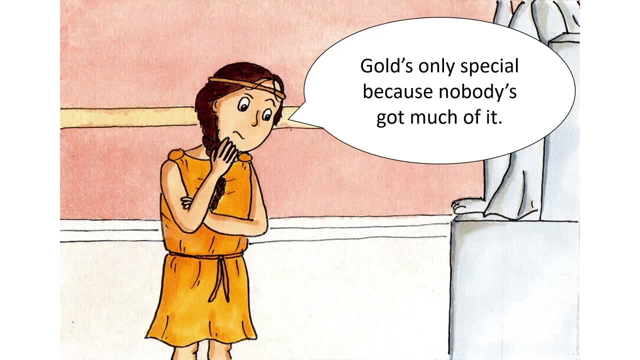 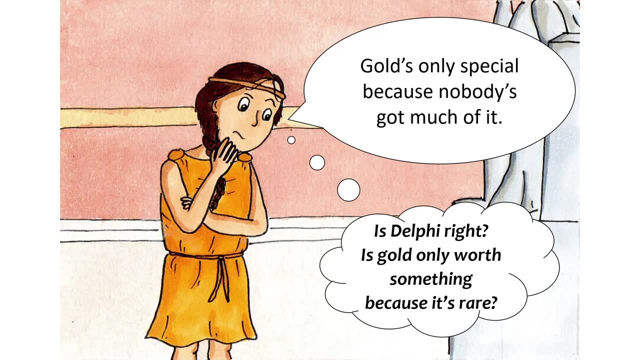 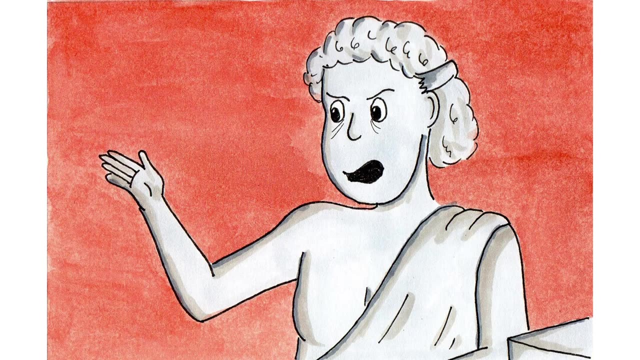 If everybody's got it, then it'll be just like anything else and it won't be worth as much. Is Delphi right? Is gold only worth something because it's rare? Dionysus almost screamed: Look, I could just smite you, you know. 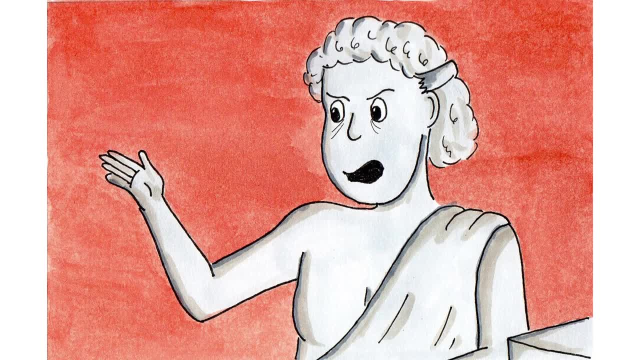 Gods aren't usually this patient, I mean. I offer you a wish for your kind—he paused. Actually, what did you do Last night's? a bit of a blur, I'm afraid. Oh, it doesn't matter now, does it? 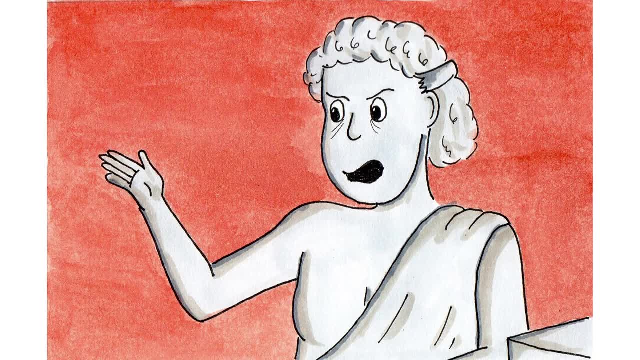 Delphi replied quickly. The god narrowed his eyes at her. She was running out of time. she knew Surely there must be something she could wish for It hit her then. She'd been so excited by the idea Being immensely rich that she had forgotten all about it before. 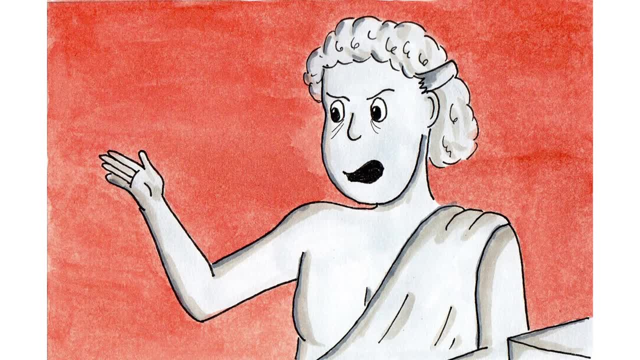 She'd been so greedy she realised her heart sinking. Why did she always have to get it wrong before she could see what was right? Just give me enough gold to free Socrates. she said: Please, That's all I want. 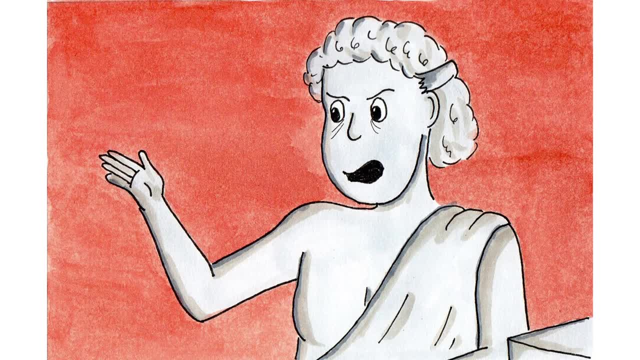 Dionysus looked up from his hands and, to her surprise, shook his head. Sorry, I'd have to give you all the gold there could ever be, and there still wouldn't be enough. What? No amount of gold will free Socrates. Dionysus said his voice soft. 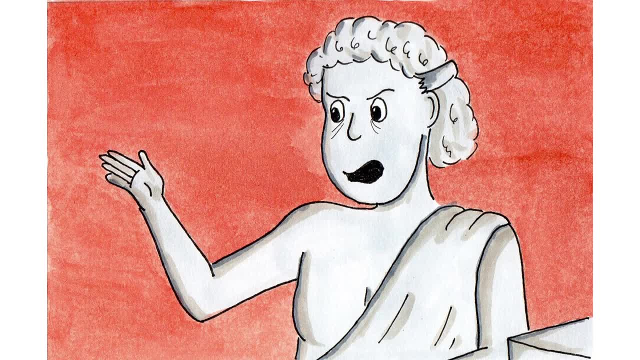 How can you buy freedom? Delphi was stunned. You mean, even if I had all the money in the world and paid all the guards and paid all the people, he still wouldn't be free. Dionysus gave her another lopsided grin. 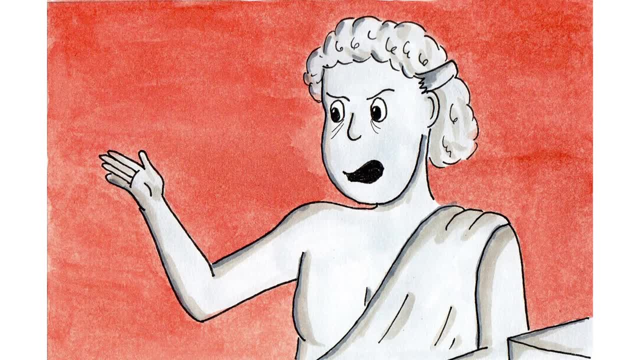 You can't buy everything. Delphi, deflated like a tired old balloon. Well, what's the point of money then if you can't do the important things? Dionysus looked rather guilty. I don't know. Giving people gold just usually ends up being a laugh, that's all. 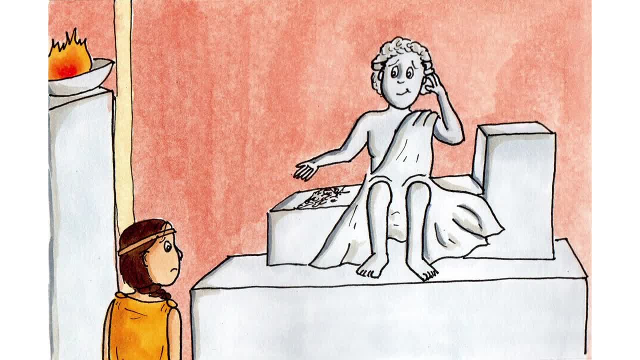 I never said it. It was a good thing. Delphi looked at the god again with fresh eyes. She realised there was absolutely nothing she could possibly ever want from him. Shall we just forget the whole thing, She suggested. Dionysus nodded enthusiastically. 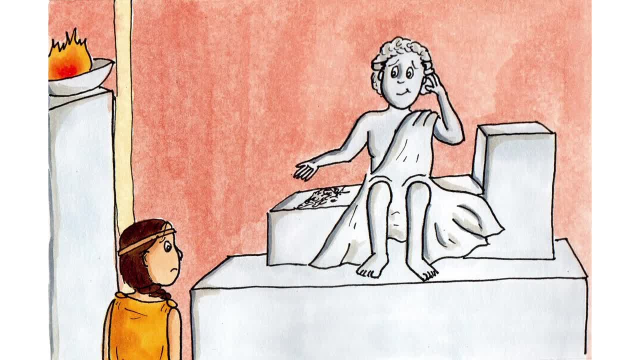 Oh would you. That would be much appreciated. The other gods get a bit funny about giving out wishes too often. Um, don't tell my dad. OK, He looked up at her, hopefully. OK, I won't, she promised. 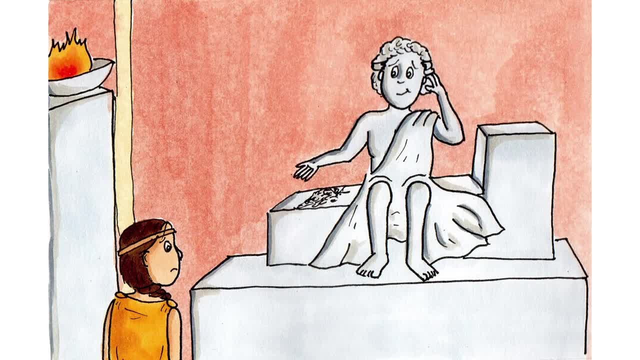 Thanks. Dionysus stood up and slowly climbed back onto the pedestal Once again, lifting the grapes up to his chest and striking a dramatic pose. Delphi was making her way out of the shrine and when she looked back, all she could see was the statue as she had found it. 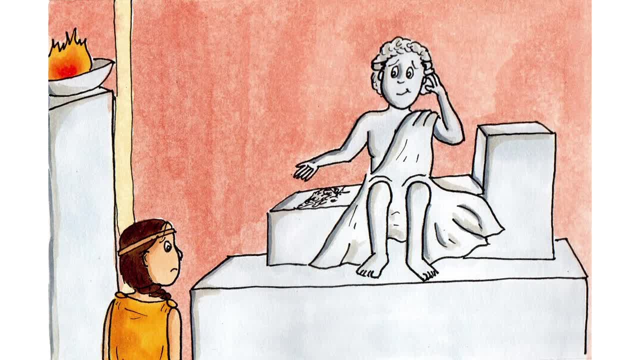 I'll bring you a better offering next time, she promised, But not money or wine. It causes nothing but trouble. She stepped out into the sunshine and was relieved to find that the trail of golden footprints had vanished. When she got home. she ate an enormous breakfast.